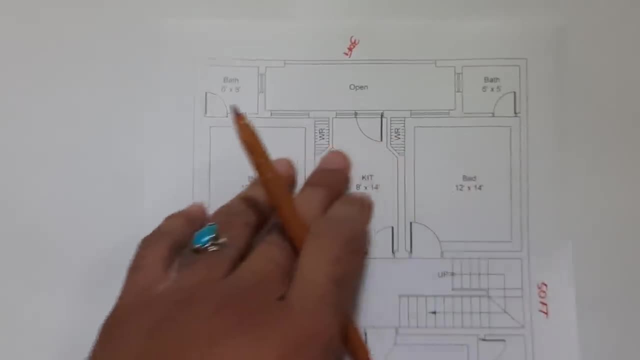 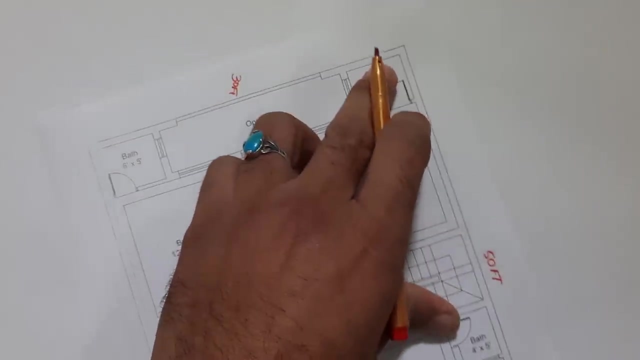 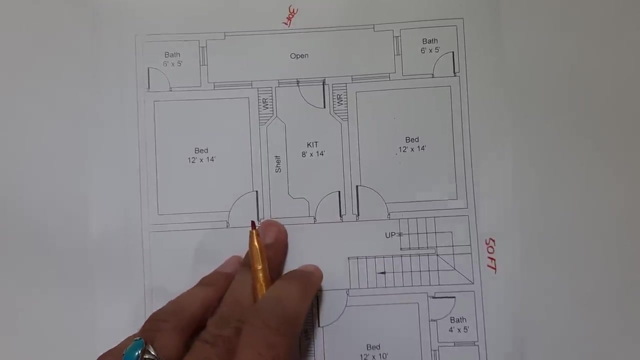 the positions of column. Guys, you can see, this is a house planning in the dimensions of 30 by 50 feet and I will show you the column positions or how to place the columns. okay, This is the topic. If you need house planning, structural drawing, 3D animation for any type of building. 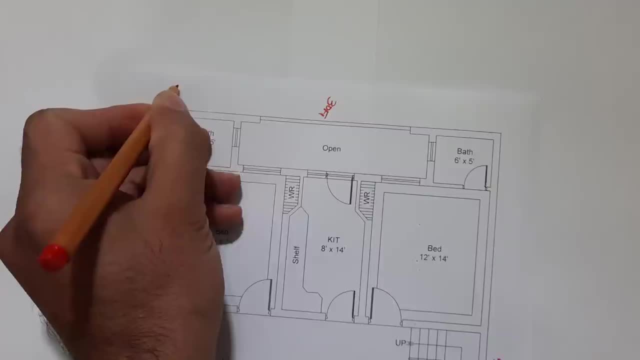 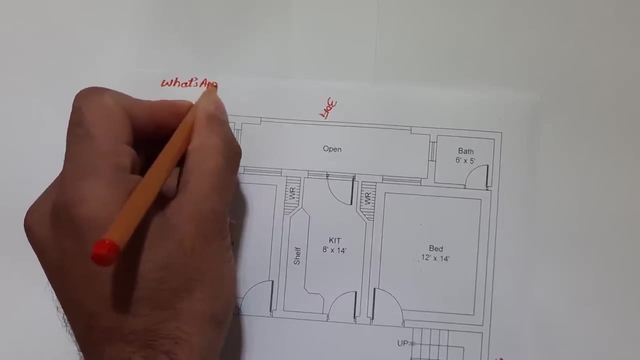 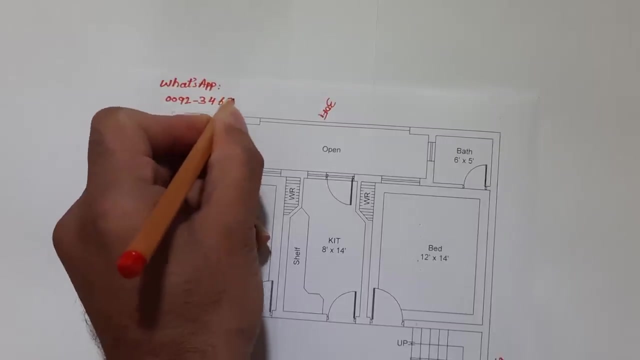 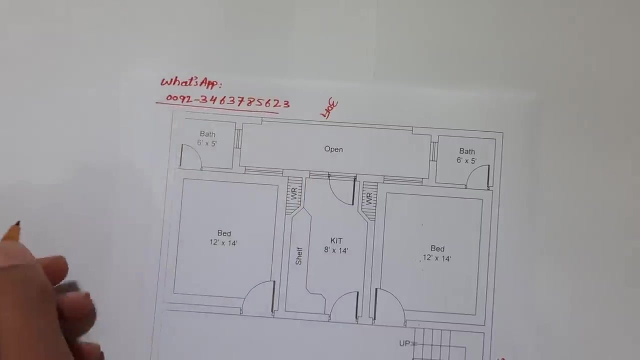 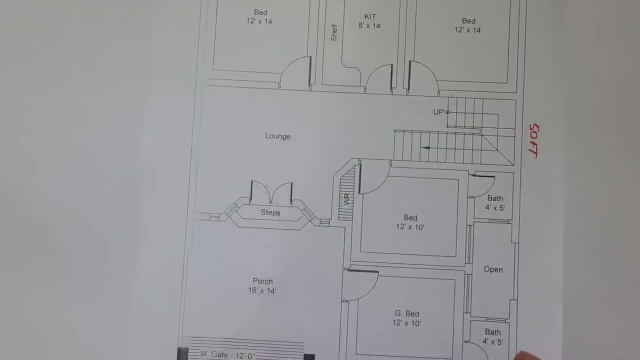 so you can contact me on this whatsapp number. This is my whatsapp number. okay, This is paid services. This is my whatsapp. If you need house planning, structural drawing, 3D animation for any type of building, so you can contact me. Let's get started, guys. This is its front side. This is road side. okay, So these two. 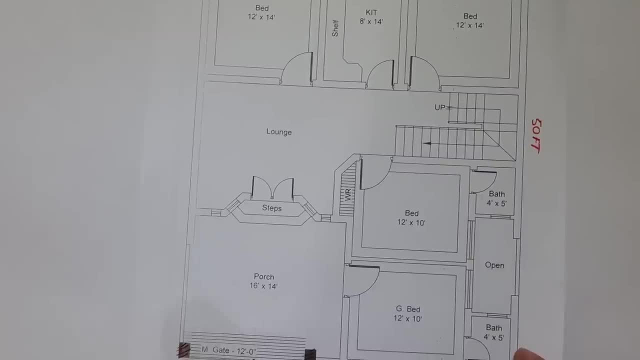 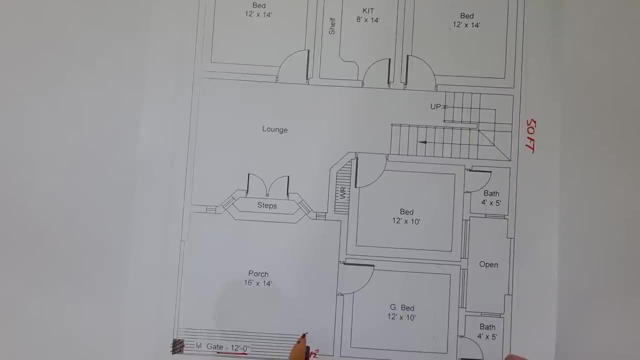 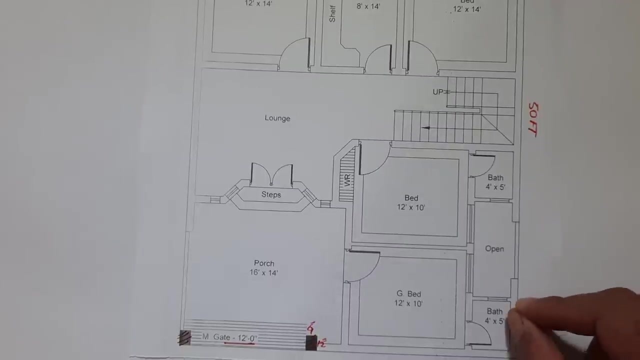 columns, guys, you can see this is for main entrance or for main gate, which width is 12 feet, okay, and size is 9 by 12 inches, okay. So let me get started from its front. Remember one thing, guys: the principles of column position is that the column should try to place. 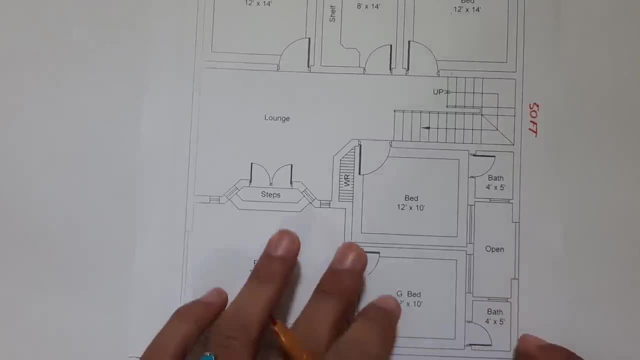 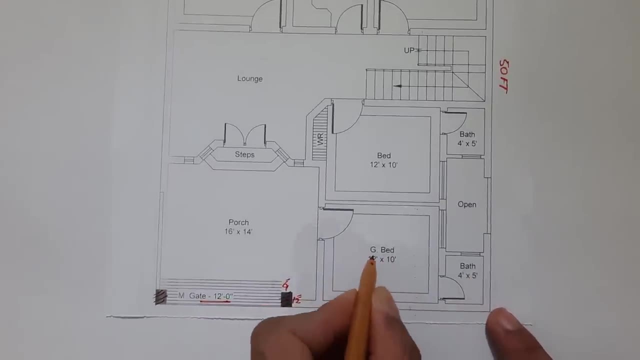 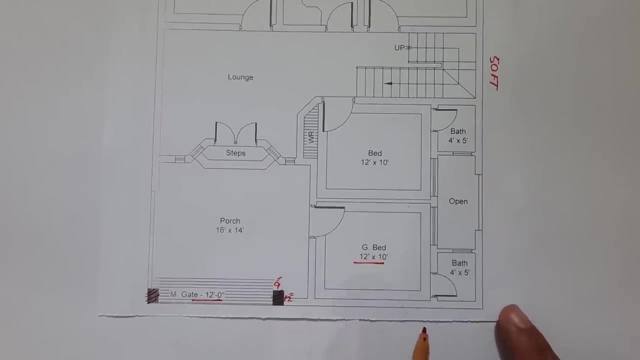 the column at the corner. okay, That will be better for you. So therefore, guys, you can see, here the first column is placing this is a bath and this is a guest bathroom. okay, Guest bedroom. okay, So size is 12 by 10 feet. So here, guys, I require to provide column at this corner, as you can see this. 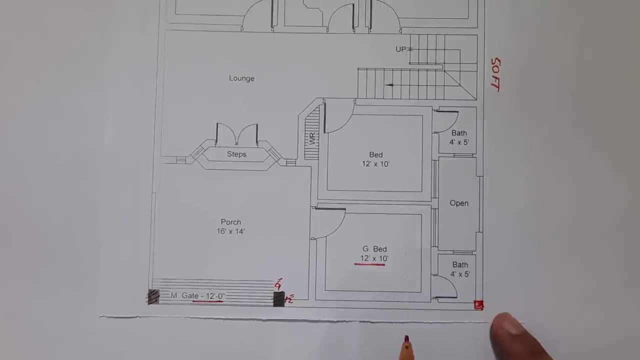 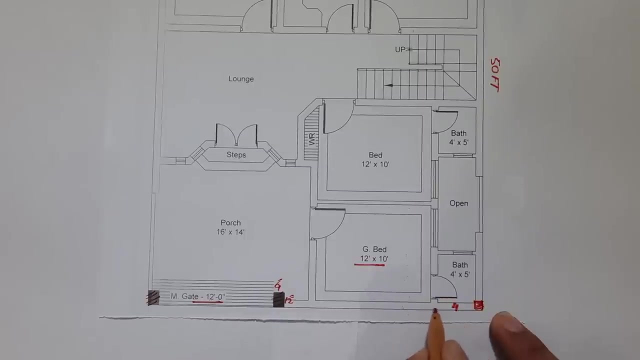 is the place to place, provide corner. next, guys, if you see, the length is 12 feet for this bedroom. okay, now, guys, you can see the bath is 4 feet, so we don't need to provide the column at this place because this is just 4 feet. so therefore we cannot provide the. 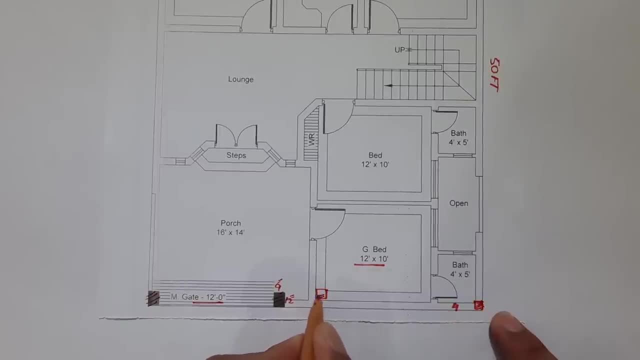 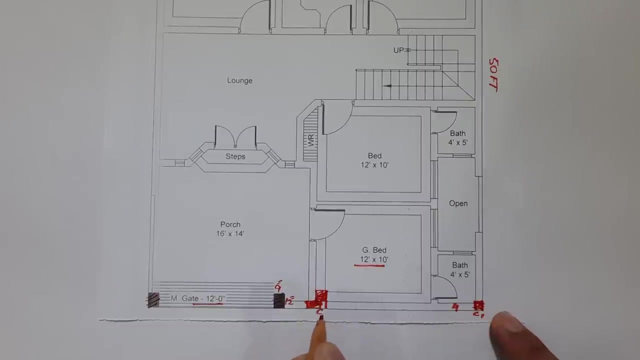 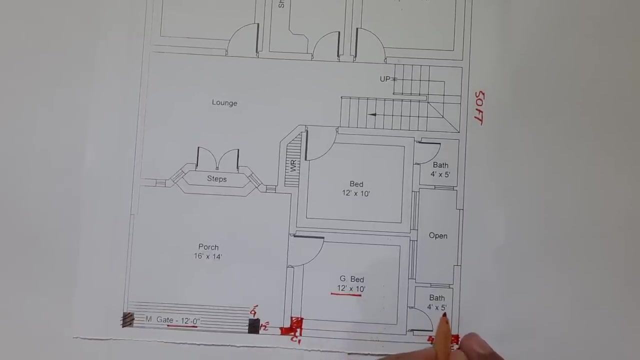 column here, so the other column should be placed at this corner of this bedroom. so these are two, sorry in this place. okay, so these are two columns. this is one column and this is the second column. see one, or you can see, see one. okay, column one. next, guys, if you see so, here the bath length is, our width is. 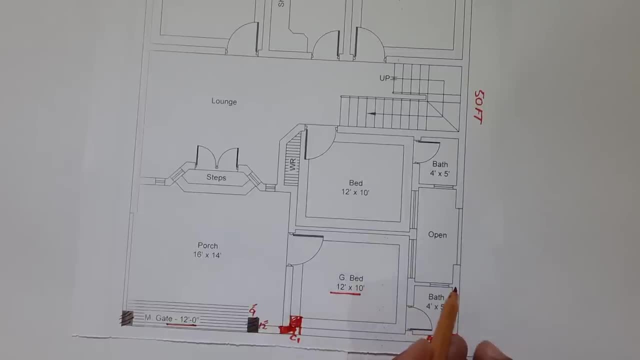 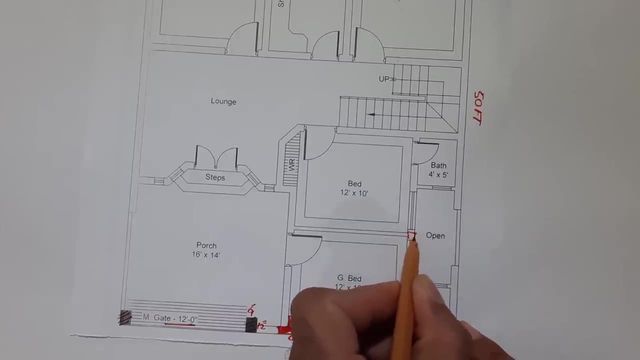 length is about 5 feet, so we cannot provide the column at this place. but here, if you see the guest, the guest bed is 10 feet, so this is the place to provide our CC column. okay, but here this is a boundary wall, if you see, guys, this. 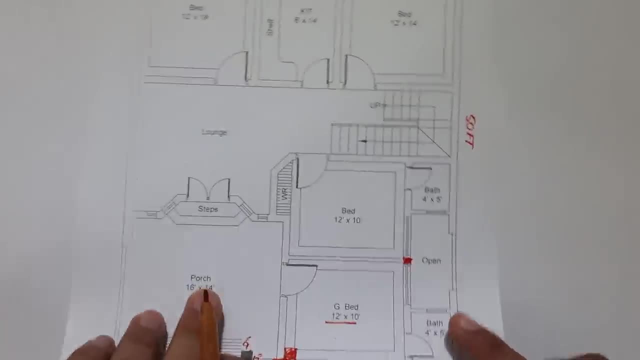 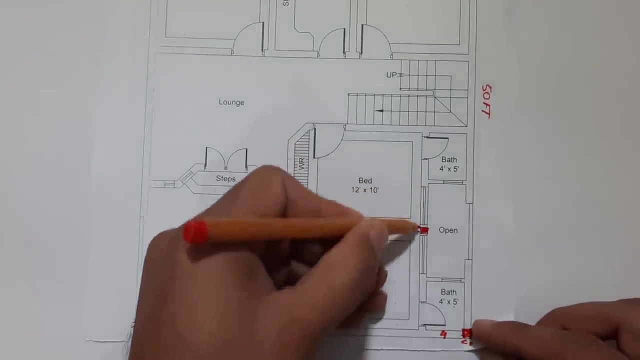 place is a boundary wall, so if you see this is a boundary wall, if you see guys is open, so if this is a boundary wall, if you see guys here, the length is about with is about 10 feet, so 10 feet, so this is going about 15 feet, so you are able. 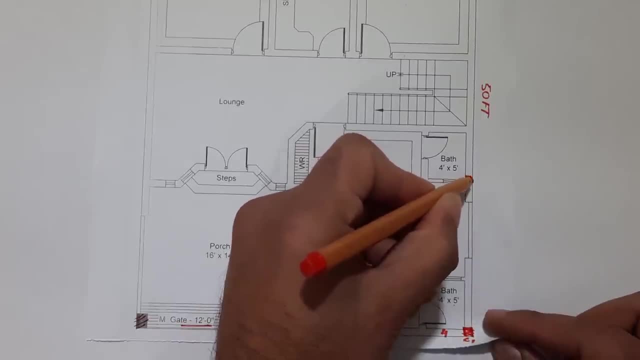 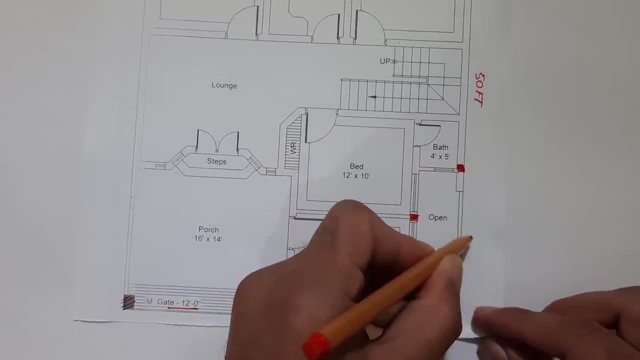 to provide the column here at this place for boundary wall. so from from 12 to 16 feet you can provide the boundary wall column, but not more than 16 feet. so up to from 12 to up to 16 feet you are able to provide the column, but the column. 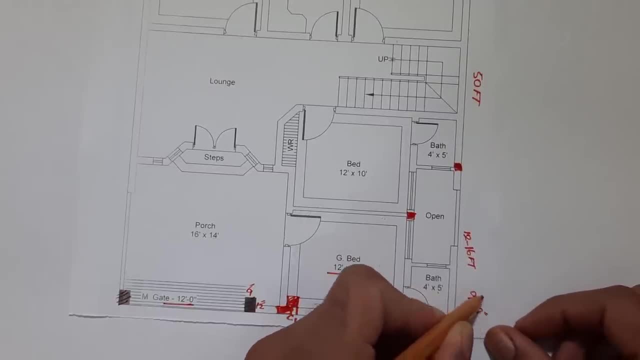 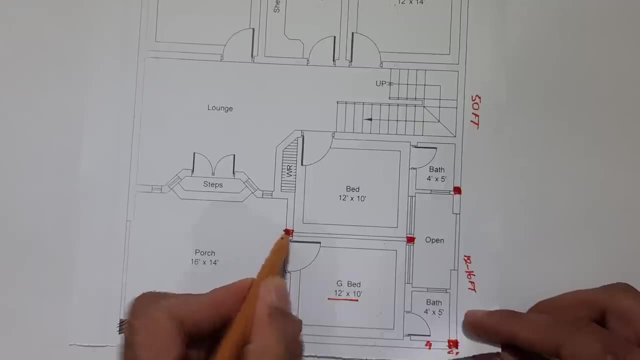 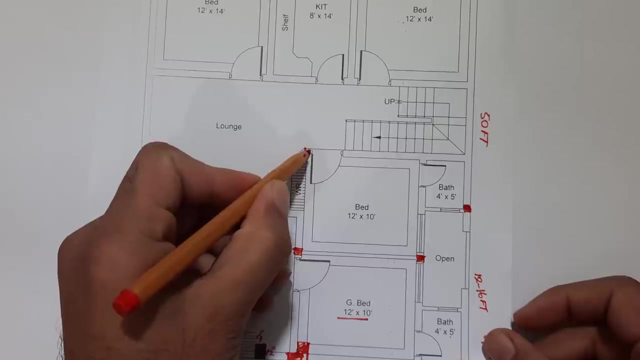 size should not be less than 9 by 9 inches, remember this. okay, so this is the column next guys. you can see this is the place to provide column at this corner. this is the other column next guys. you can see this is the place to provide the column at this corner. okay, next guys, i will provide. this is just ground. 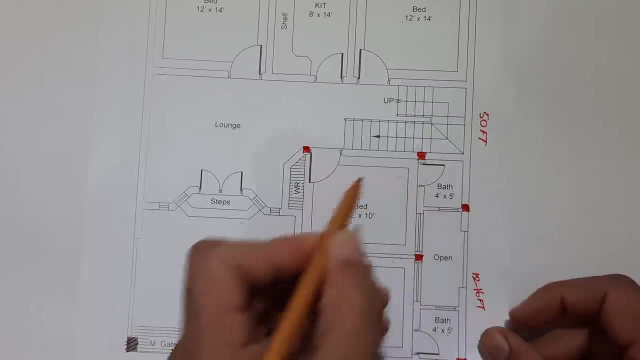 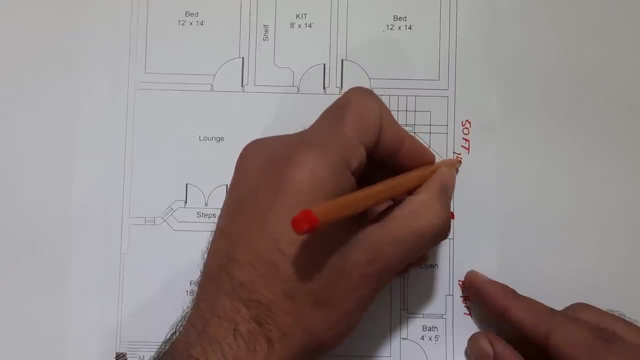 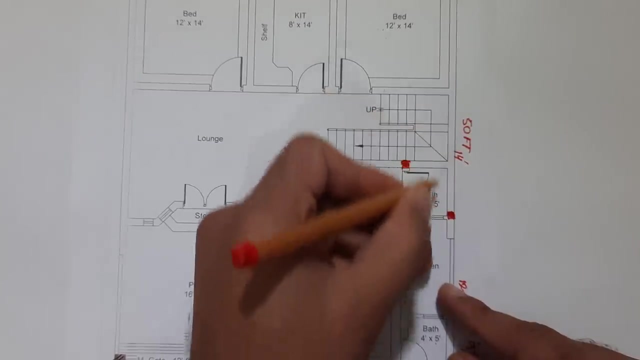 floor plan. okay, you can provide the column here. okay, so here we don't require, because the length is here about 14 feet for this tier and also for this one. okay, so sorry, not 14 feet. so this is about 12 feet, this is 7 feet and this is 5 feet, so this is just 12 feet. 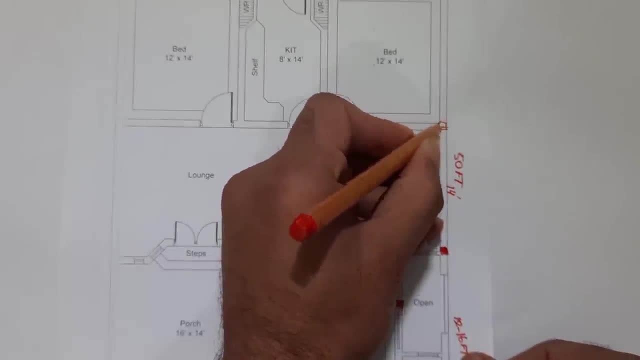 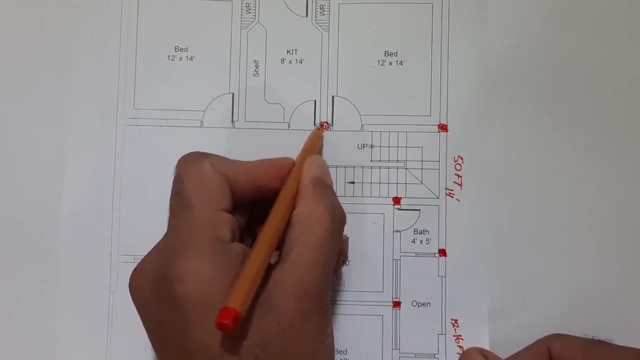 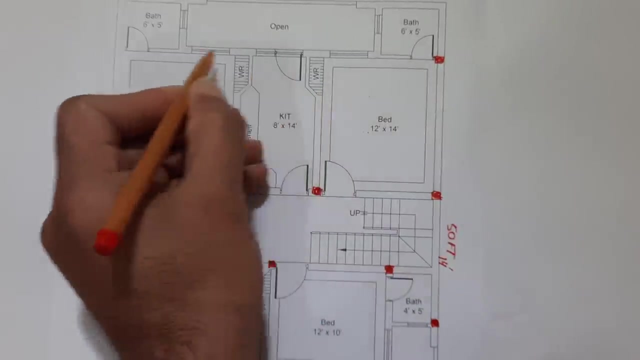 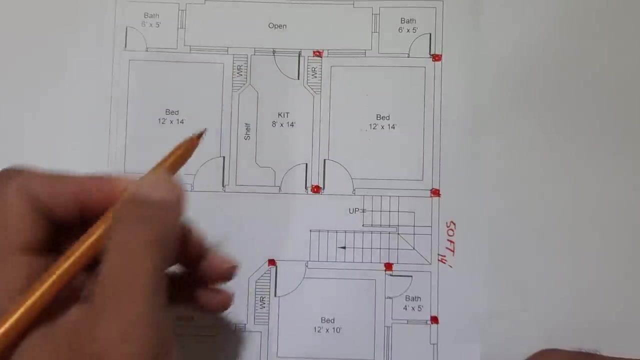 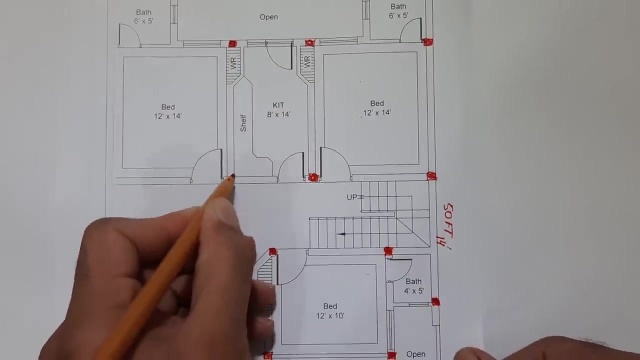 so the next column you can provide at this corner, okay. next one, guys, you can place at this place for this bedroom. okay, the next one you can provide here at this place. next one you can place here. next, you can place here, because width is 8 feet. next one you can place here. 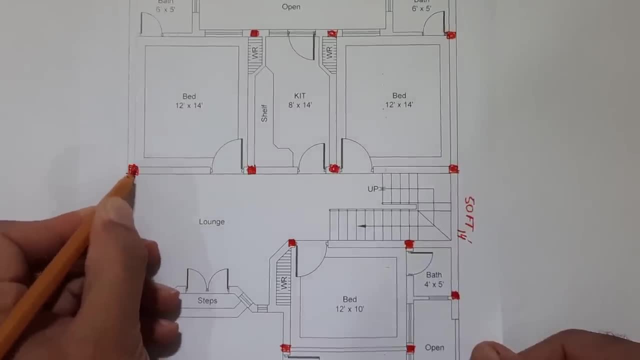 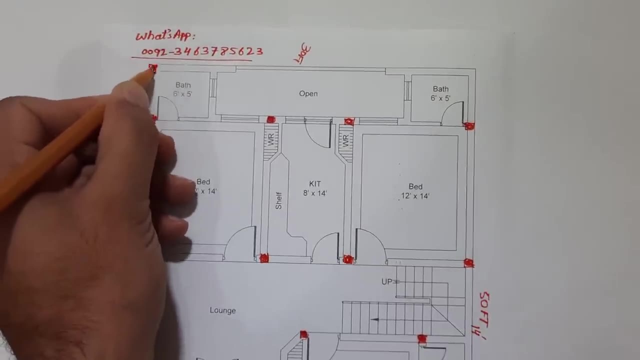 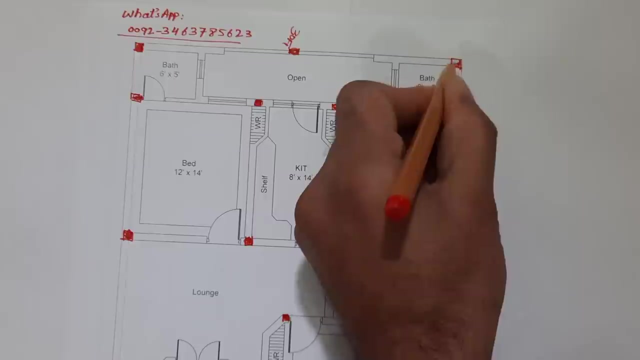 okay, this is the corner for this bed you can provide here. this is the other one you can provide here. this is the corner, boundary corner, so important to provide here. this is 30 feet, so provide the middle one here. this is the other one corner you can provide here. okay, now come here, guys. this is the tv launch.